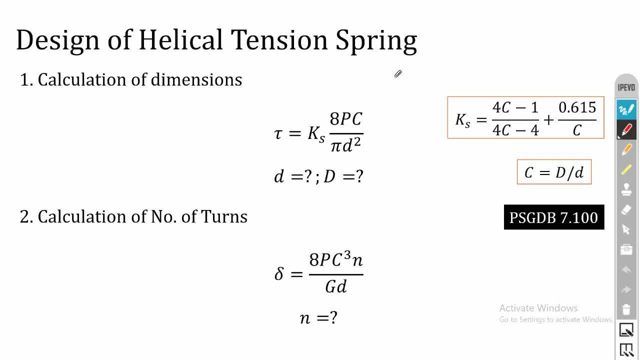 of turns and calculation of free length. So the remaining procedures are same. So the first step is calculation of dimensions. So in the problem they will specify the shear stress of the material and the spring index and load value. So by substituting the value 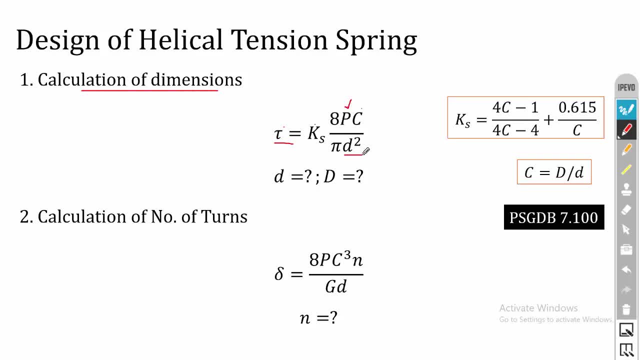 of tau kspc, we can calculate the diameter of the wire and we know that the spring index c is the ratio between coil diameter and wire diameter. So by substituting the value of d in the c equation we can calculate the capital D. So after calculating the diameter of the spring, then the second step is calculation. 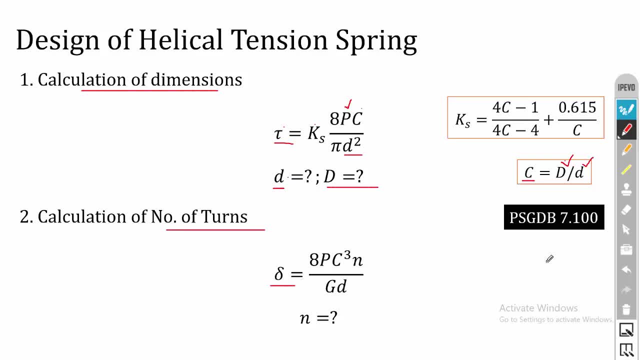 of number of turns. So this equation is also there in the data book, page number 7.100.. Del is equal to 8pc3n divided by gd. Here del is the deflection, p is the load, c is spring index, n is number of turns, g is modulus of rigidity and d is the wire diameter. So 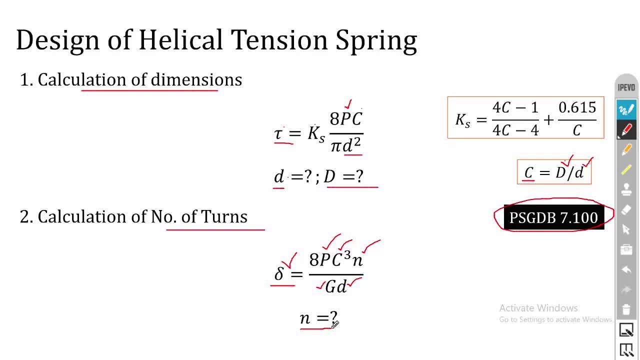 by substituting the value of tau kspc, we can calculate the diameter of the wire, and we know that the spring index c is equal to 9pc3n divided by gd, which is number of turns. Now we can calculate the total number of turns. Then, after calculating the number of turns, 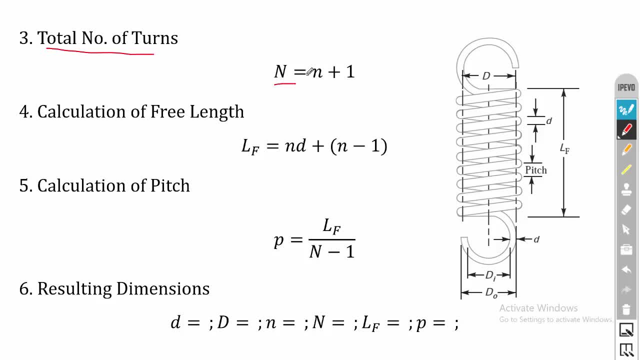 we have to calculate the total number of turns. So for all the helical tension springs the end conditions are same. So the end is a curved like structure. N is equal to n plus 1. So it is common for all helical tension springs. Then calculation of free length, lf, is equal. 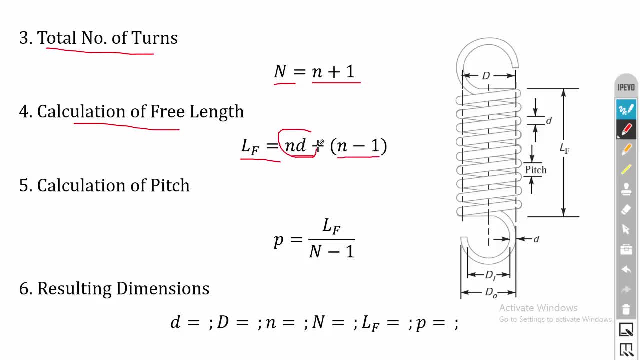 to nd plus n minus 1.. Here n is the small n, that is total number of active coils. So n into d plus n minus 1.. So this is for the clearance. Then, finally, the calculation of pitch P is equal to LF divided by n minus 1.. 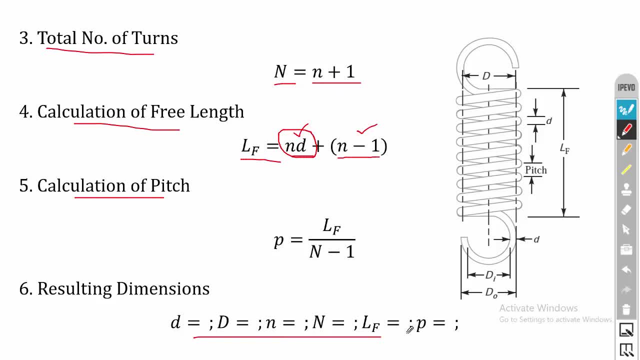 So after calculating all the dimensions we can write everything as a resultant dimensions. So this is the drawing for helical tension spring. So this is the coil diameter and small d is the wire diameter, di is inner diameter and do is outer diameter. The distance between adjacent coils is called as pitch and the length of the spring at the 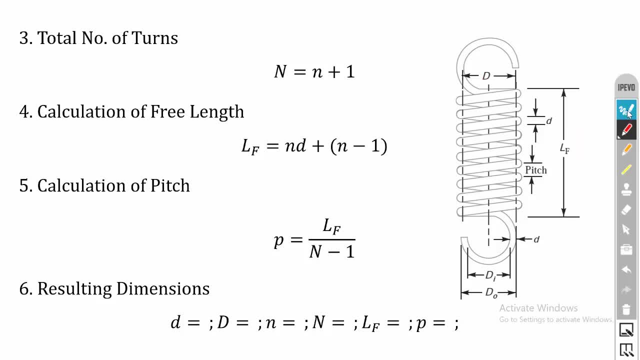 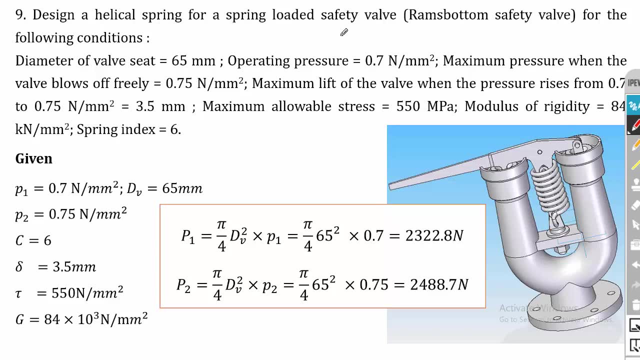 elongated state is called as free length. So the first problem: Design a helical spring for a spring loaded safety valve. This is called rams bottom safety valve, So remember that the technical term rams bottom safety valve. So this is the rams bottom safety valve. 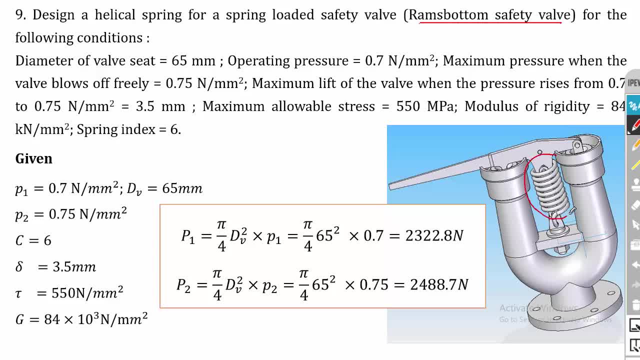 So this is the structure and here in the rams bottom safety valve that helical tension spring is used. So whenever in the problem if you see the word rams bottom safety valve, then we have to select the helical tension spring, not the helical compression spring, because there will 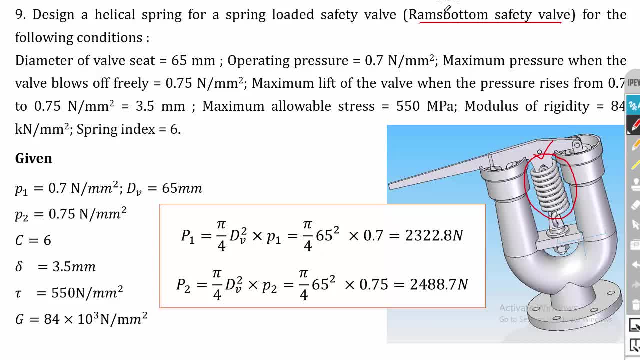 be no difference in the problem. So only thing for rams bottom safety valve. Ok, For rams bottom safety valve we have to use the helical tension spring. So the diameter of the valve seat is 65 mm, The operating pressure is 0.7 Newton per mm square. 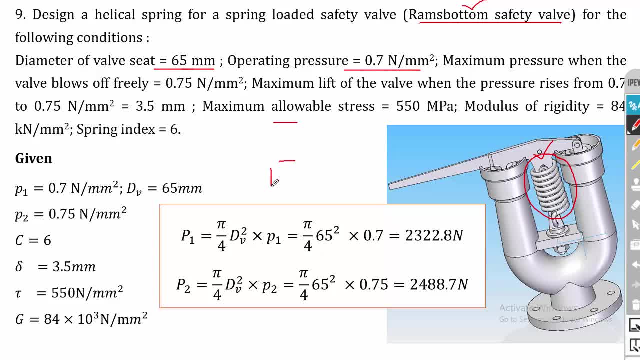 So here we have two pressure values. The first one is operating pressure, that is P1.. So, just like the pressure relief valve design, Then maximum pressure when the valve blows off freely, Ok, So So after reaching the 0.7 Newton per mm square, what will happen is the valve starts to blow. 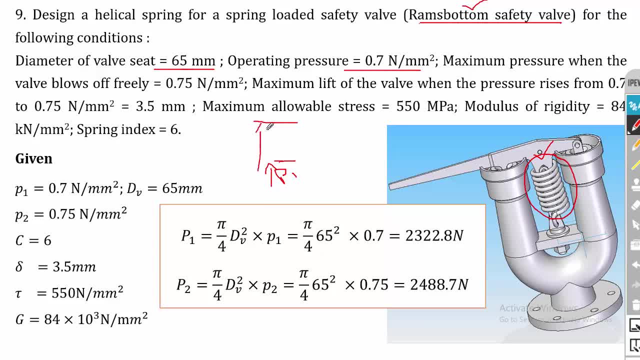 off. Ok, So after reaching high pressure of 0.75, the valve is completely opened. Ok, So the valve is completely opened. Remember that the valve starts to open at a pressure of P1 and it is completely open at P2.. 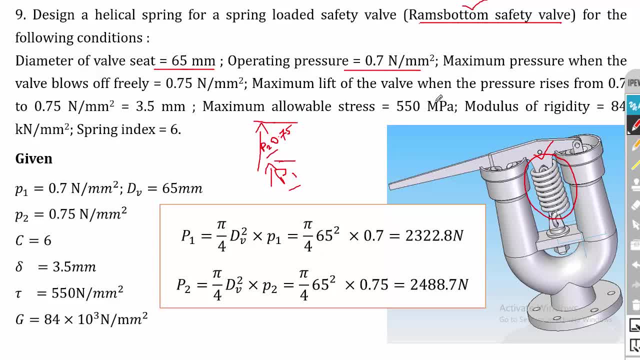 Ok, The maximum lift of the valve when the pressure rise from 0.7 to 0.7.. Ok, 0.75 Newton per mm square is 3.5 mm. So this lift from 0.7 to 0.75 is 3.5 mm. 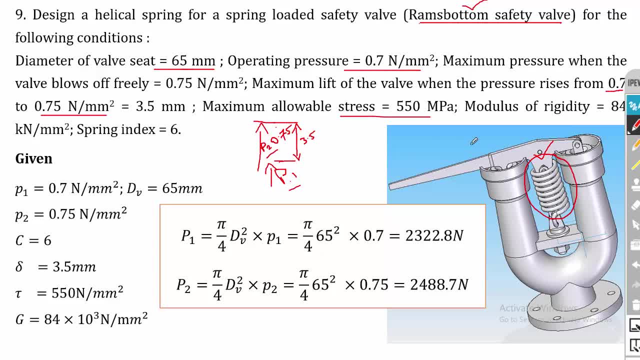 Ok, So the maximum allowable stress is equal to 550 MPa and the modulus of rigidity is equal to 84 kN per mm square. that is, 84 into 10 power 3 Newton per mm square. Then the spring index is given as 6.. 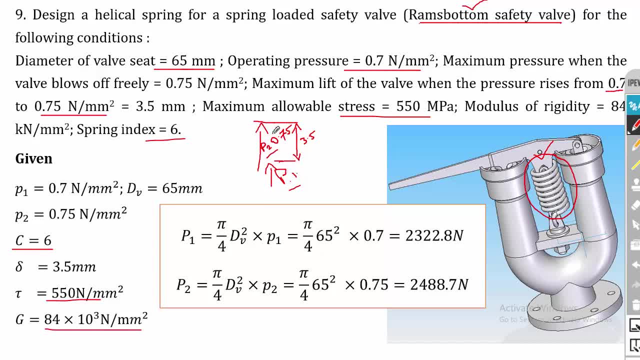 Ok, Then the problem. the P1 value and P2 values are given. So by using the P1 value and the diameter of the valve dv value, we can calculate the load 1 and load 2.. And this 3.5 mm is actually the lift, that is the deflection from P1 to P2. so it is del. 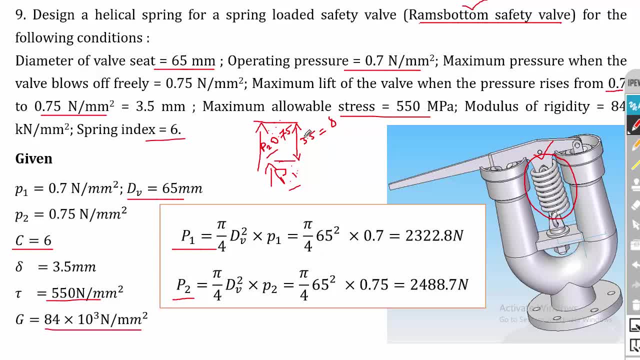 So 3.5 is equal to del. So we have already solved this kind of problems earlier. So you know what is the meaning for del, That is, That is the deflection from P1 to P2.. So in the case of helical compression spring, it is compression, and in the case of helical 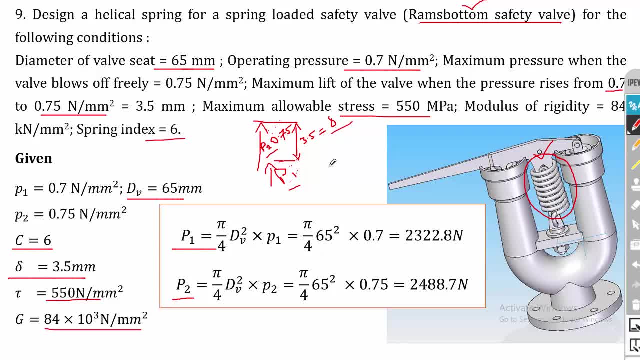 tension spring. here it is the elongation. So del is equal to 3.5 mm is the elongation of the spring. So we will calculate the P1 and P2 first. So P1 is equal to 5 by 4 dv. square into small p1, substitute the value of dv and p so that 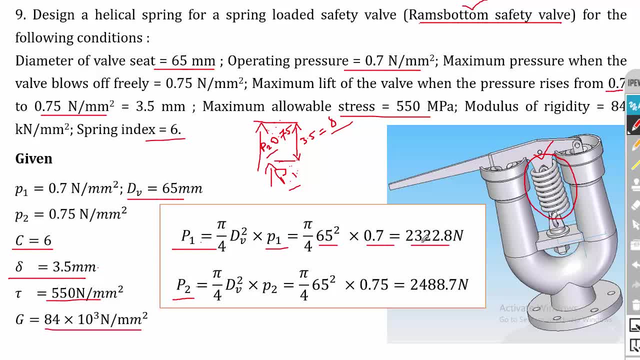 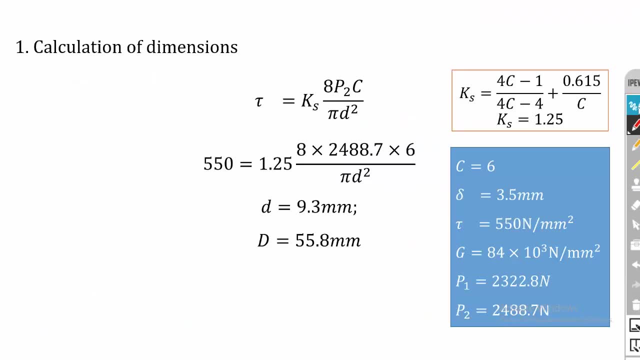 the maximum, I mean the minimum pressure is. minimum load is 2322.8 newton. Then for maximum load substitute the maximum pressure value. it is 2488.7 newton. So after calculating the P1 and P2 value, we can start the design procedure. 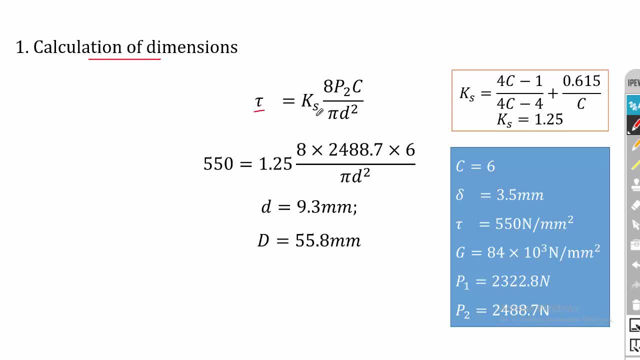 So the first step is calculation of dimensions. So tau is equal to Ks 8 P2.. We know that for calculating the shear stress We have to use the maximum P value. So if there is only one P value in the problem, then there is no confusion about that. 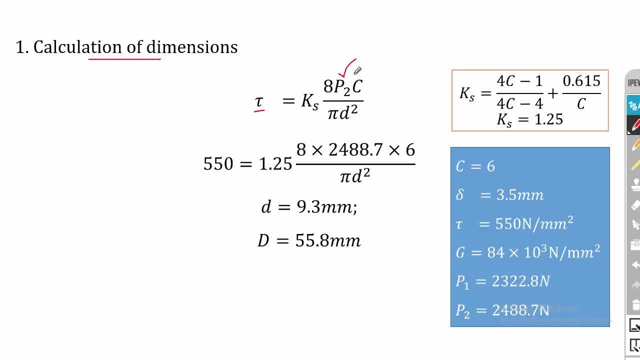 But when you have two load values, that is, P2 and P1, you have to be very careful And for calculating the shear stress you have to select the maximum load. So it is Ks 8, P2 C divided by pi d square. 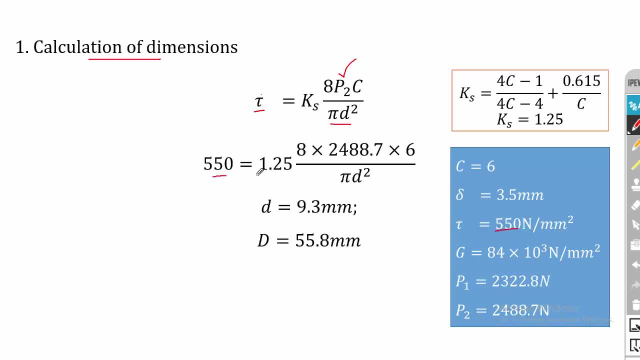 So tau value is given. in the problem it is 550. you can substitute that. Then C is given as 6.. So the equation for Ks Ks is 4C-1 by 4C-4 plus 0.615 Divided by C. 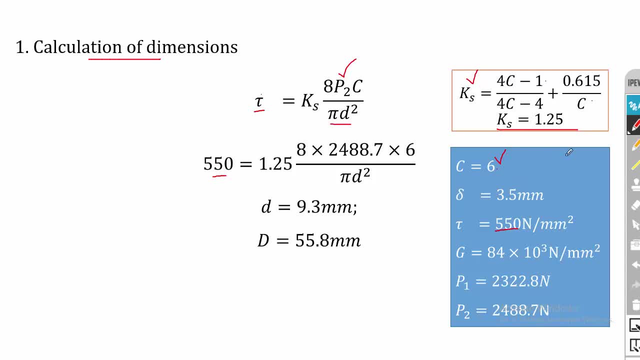 Substitute the values of C in this equation so that you will get: Ks is equal to 1.25.. So now you can substitute the value of Ks here and C and the maximum load. So by solving this equation you will get the diameter of spring. ie wire diameter is 9.3mm. 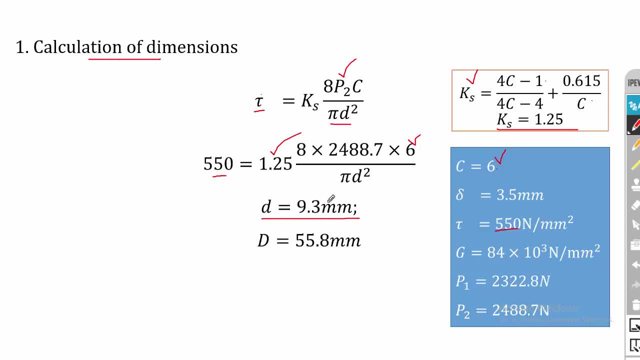 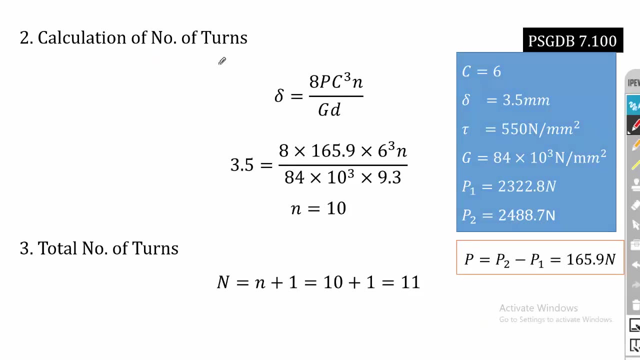 P. the wire diameter in the CE equation, that is C, is equal to capital D by small d so that you will get the coil diameter. D is equal to 55.8 mm. The second step is calculation of number of turns use. the equation del is equal to 8p. 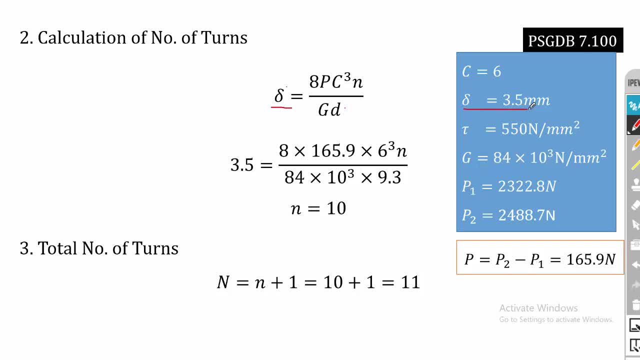 C cube N divided by GD. so del, it is directly given. it is 3.5 mm and P. so we know that we have two load values. one is P2 and the other one is P1. so the valve starts to open at P1 and it is completely open at P2. so this distance is deflection del. so when you are substituting, 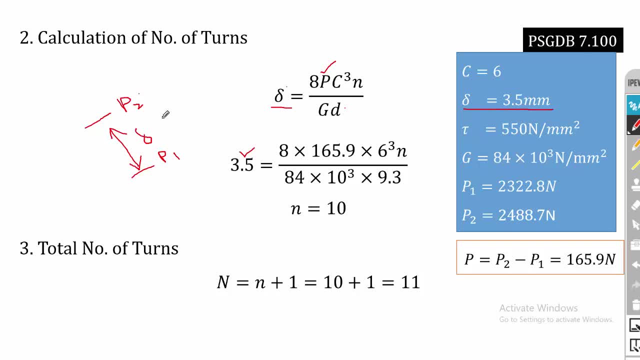 the del in the number of turns equation you have to substitute the P value, that is load range for this amount of deflection. so what is the load range for del deflection? and we know that P is equal to C, P2 minus P1, so it is very important. so P2 minus P1. P2 is given, P1 is given, so P2 minus. 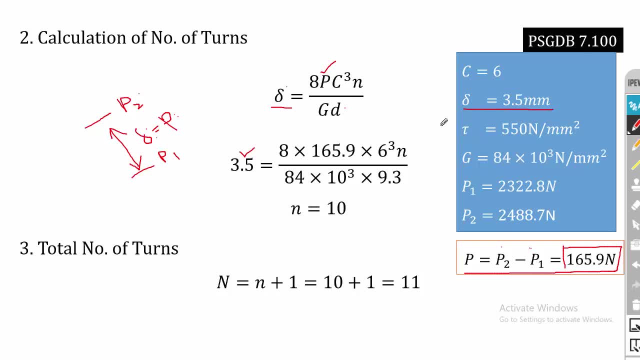 P1 is 165.9 N. so substitute everything in this equation and calculate the N value. N is equal to 10 turns, so small n is actually the number of active coils. then the total number of turns for helical tension spring is capital. N is equal to N plus 10.. 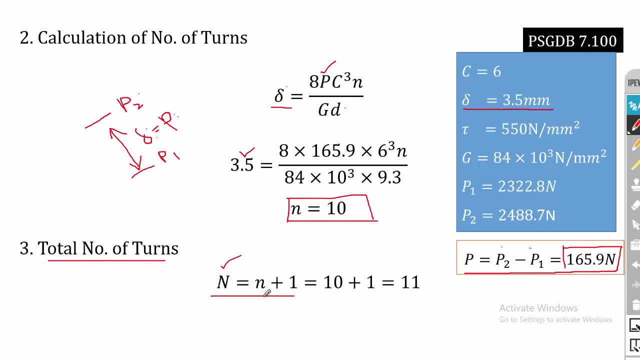 N is total number of turns, including active and inactive turns. so the difference between active and inactive turns is the active turns will carry the load and the inactive turns will not carry the load. so in general the inactive turns are at the inside. so here the active turns is 10, so it is 10 plus 1, that is equal to 11.. 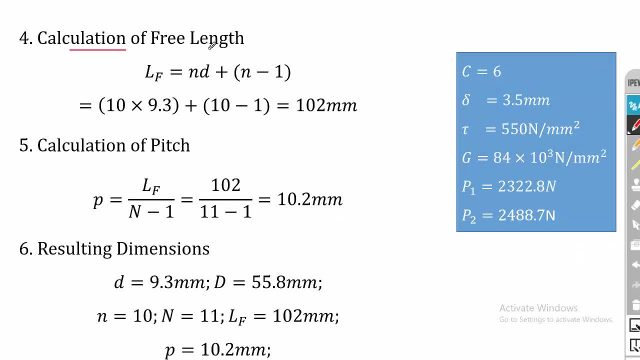 Then the forth step is calculation of free length. and free length for a helical tension is: lf is equal to nd plus n minus 1, so we have all the values. substitute it, you will get 102 mm. then pitch p is equal to lf divided by n minus 1, so it is 10.2 mm. so the last. 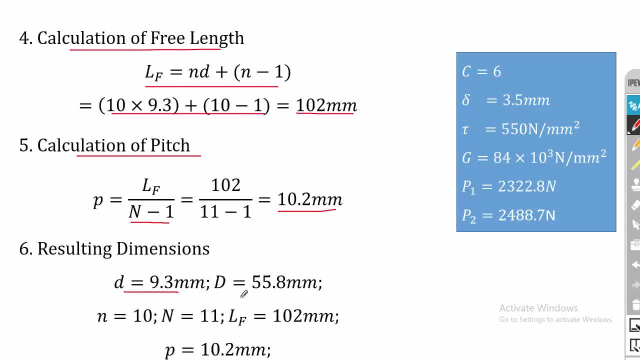 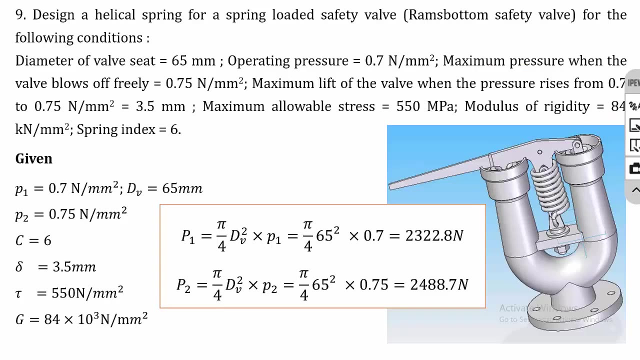 step is resulting dimension. write all the calculated dimensions in the final step. ok, so this is the design procedure for helical tension spring. so there are two differences. one is the total number of turns and another one is calculation of free length according to this problem. remember that in rams bottom safety valve, helical tension spring will be. 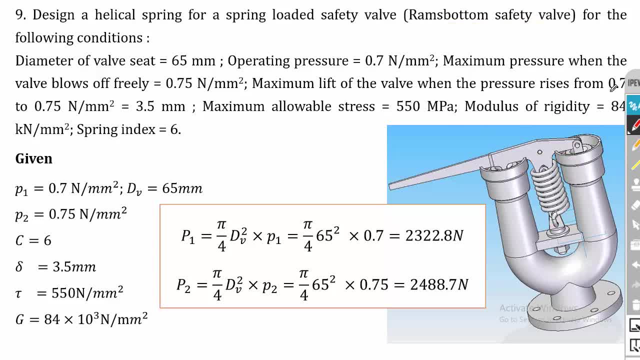 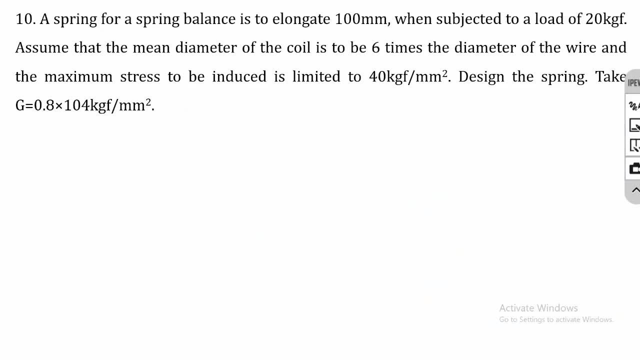 used. ok, it is not helical compression spring. so be clear about it, because in the problem they haven't specified anything about helical tension spring or helical compression spring. ok, so the only key word is rams bottom safety valve. so the tutorial problem- a spring for a spring balance- is to elongate 100 mm. ok, so here the 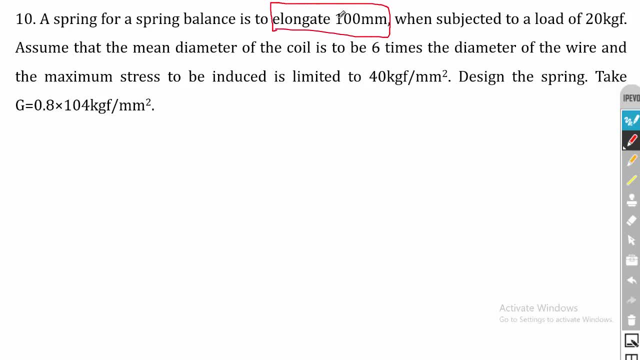 spring is used to elongate. elongate means it is providing some. it is capable of carrying tensile load. ok, so the del is 100 mm and the meaning for elongation is here. the spring is a helical tension spring. ok, so it is not compression spring, because the compression spring will not elongate the compression. 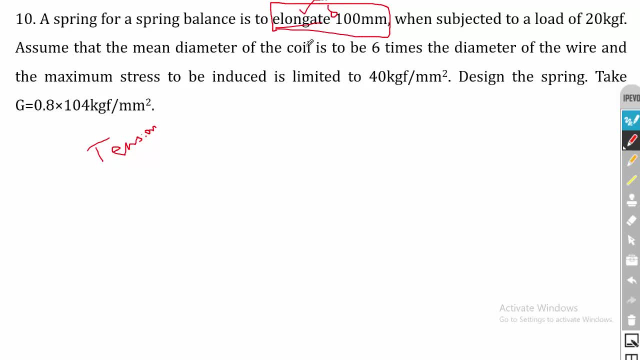 spring will compress, the tension spring will be elongating. ok, so here. the spring is a helical tension spring when subjected to a load of 20 kgf. so it is actually given in kgf. you can convert it into newton by multiplying 9.81. assume that the mean diameter of the 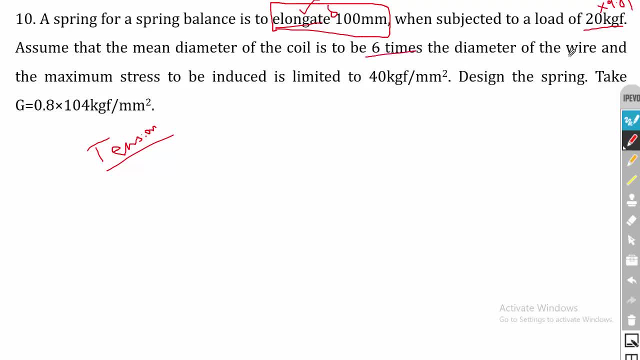 coil is to be 6 times the diameter of the wire, so the meaning is capital. d is equal to 6 times the wire diameter, so c is equal to d, because d by d, you will get 6. the maximum stress to be induced is limited to 40 kgf per mm square, so tau is